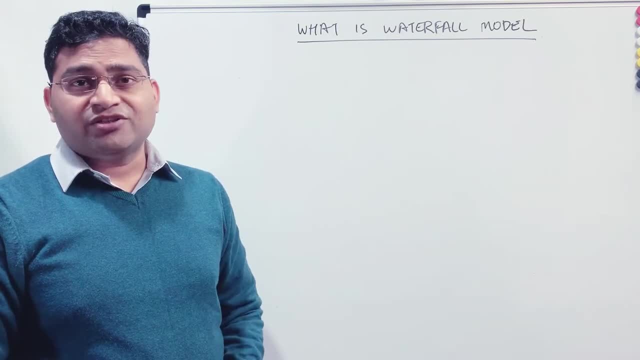 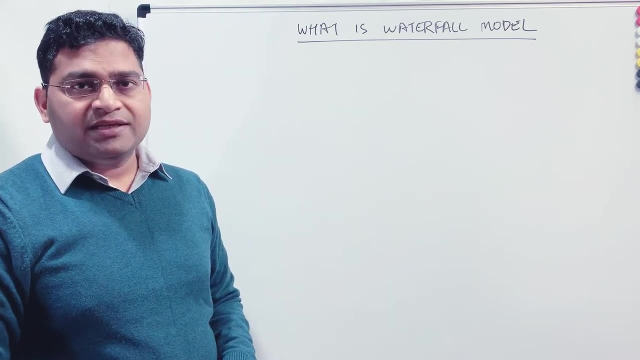 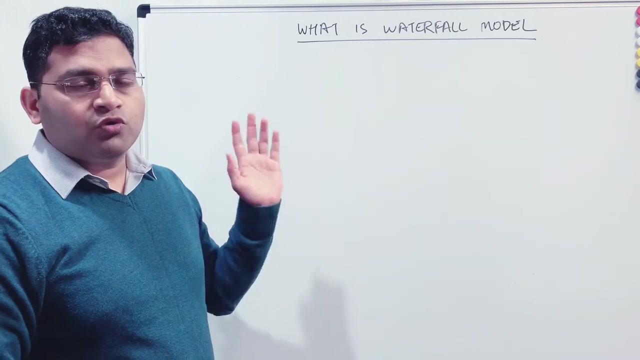 Hello everyone, welcome again. In this software testing tutorial we are going to learn what is waterfall model. So in the previous tutorial we have already seen about the software development life cycle. Now let's understand what is waterfall model or waterfall development approach. 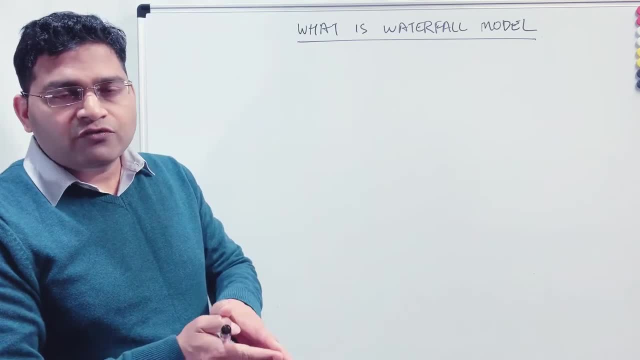 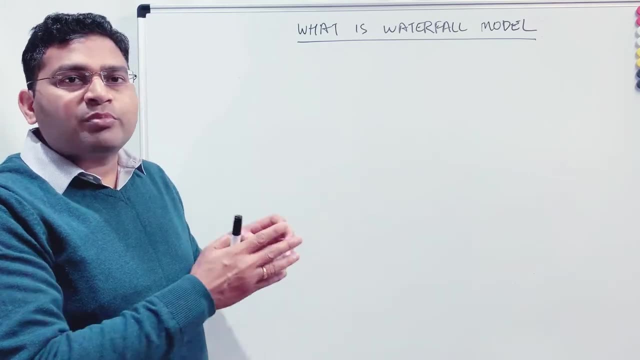 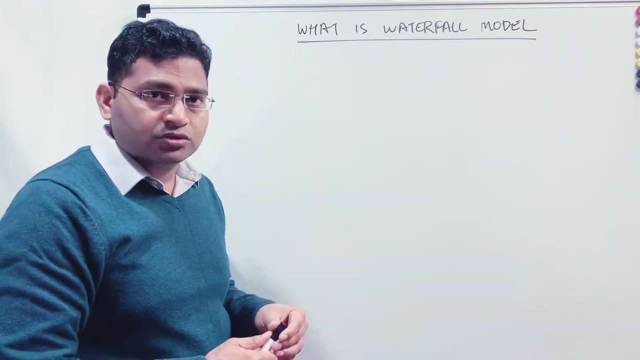 Now, as we have understood about the software development life cycle, waterfall approach is a software development life cycle or it follows very similar phases or process, as we have understood in the software development life cycle. Now let's understand how the waterfall model looks like. So in the waterfall model, the process is something very similar to what we have. 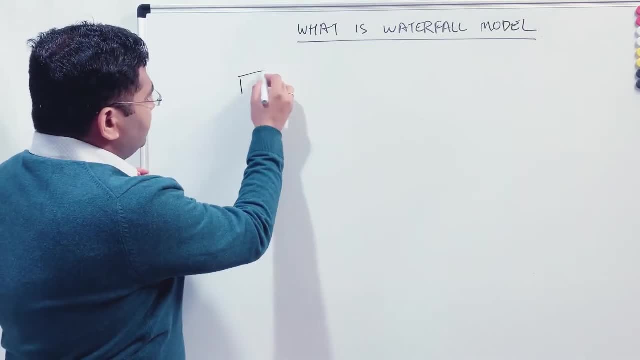 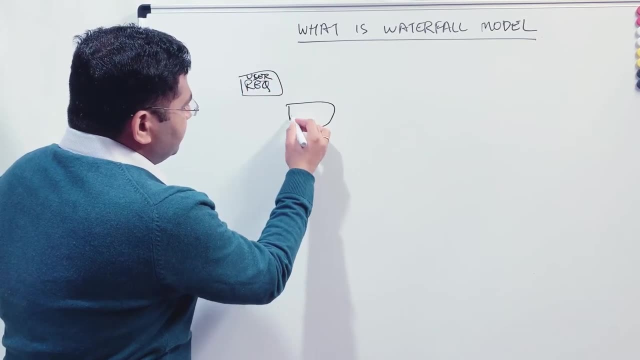 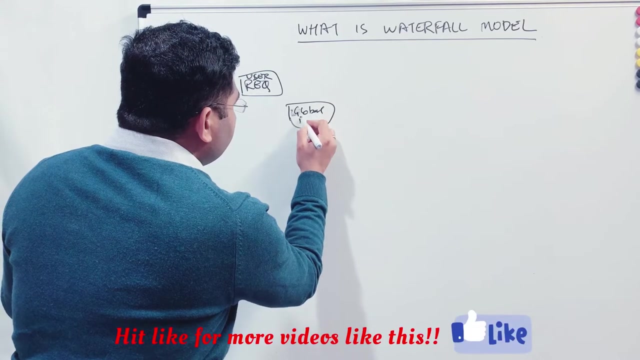 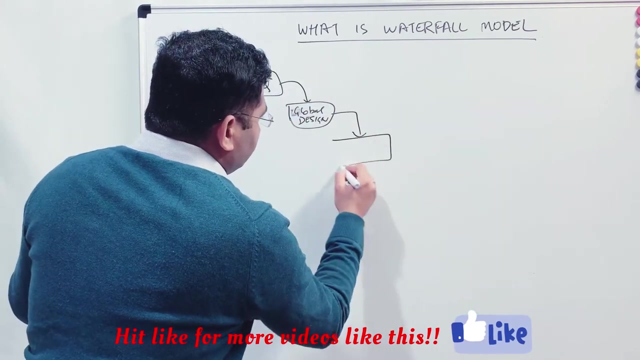 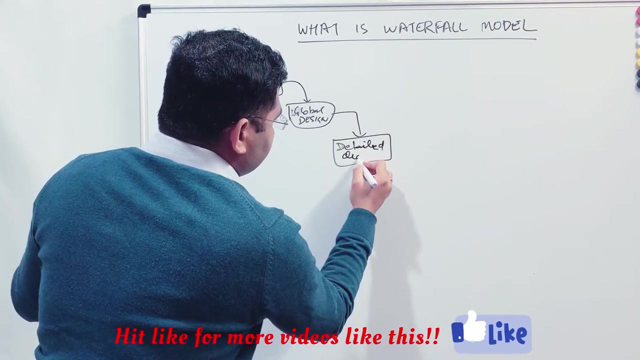 seen in software development life cycle. So the first phase is the requirements phase, or requirement gathering phase, So user requirements. The next phase is the global design, So global design or high level design. Okay. The next phase is detailed design, Detailed design. Once the detailed design is done, then you have the coding phase. 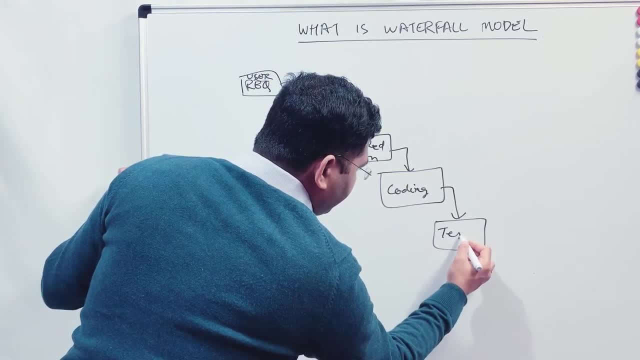 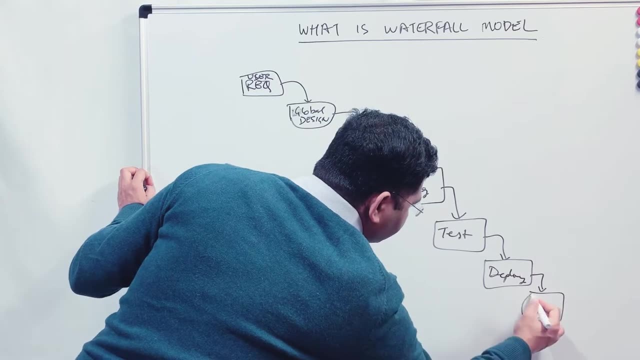 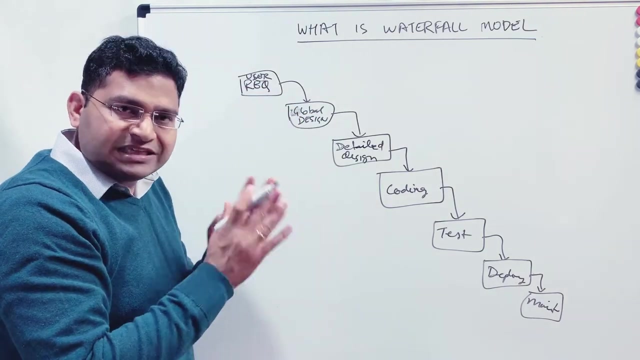 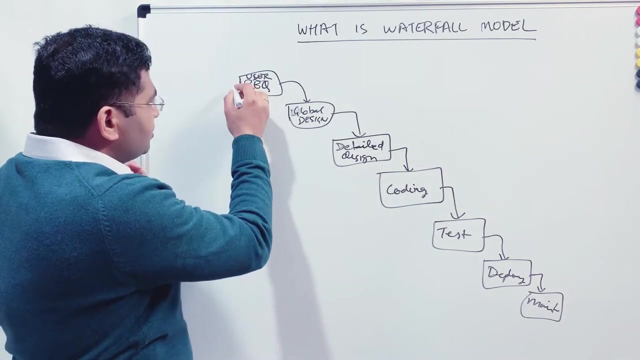 Then you have the test phase, Then you have deploy, So deploy to production, And then you have maintenance. Okay, So this is the usual workflow, or the process that teams, development teams, follow when they are following the waterfall model, waterfall development approach. Now, if we talk about this flow, 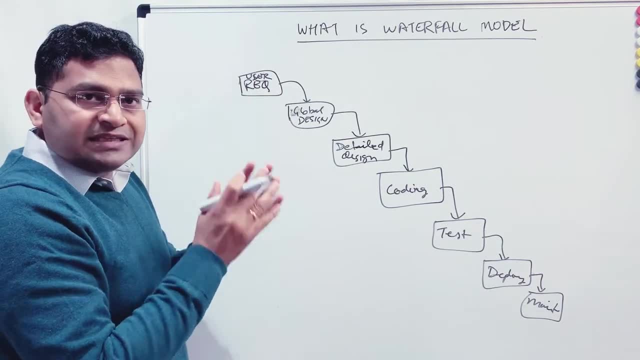 basically so user requirement is the phase wherein the team or the development team that is developing the software- So the development team that is developing the software, So the development team that is developing the software. there will be a few people who will be working in. 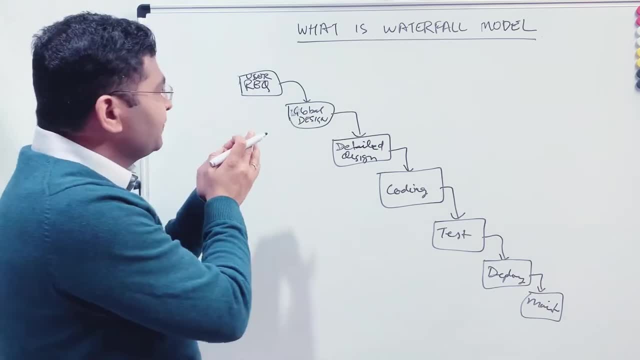 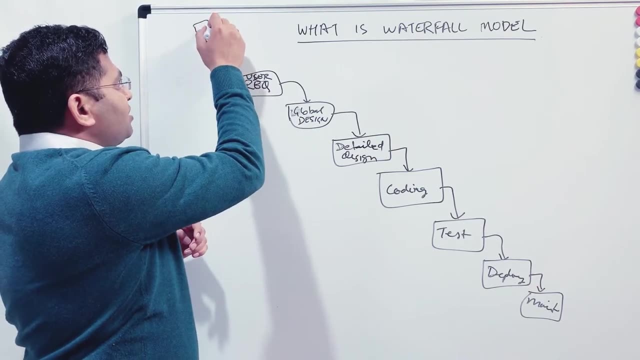 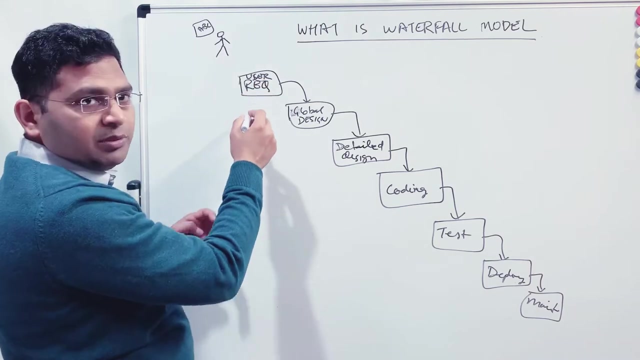 the user requirement or product management space. who will gather the user requirement from the customer? Okay, So, for example, this person is the customer, He'll be representing some of the organization ABC right, And there'll be a person or group of people who will provide the requirement. 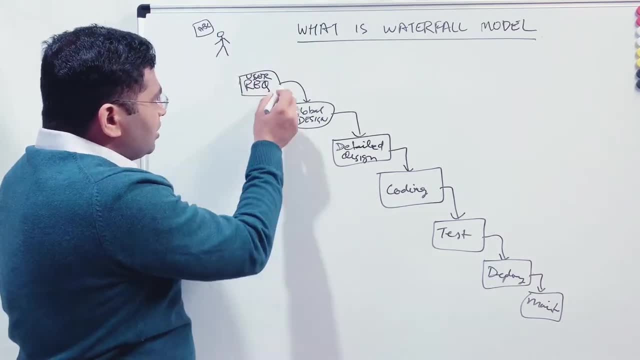 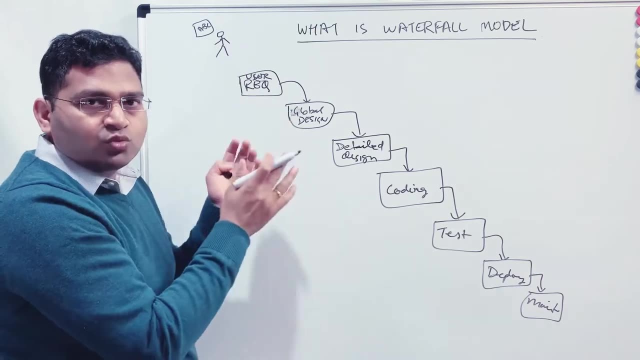 for the particular software they are trying to build. Okay, Those requirements will be gathered. once the requirements are being gathered and analyzed and finalized and signed by the customer- Yes, this is what we want- Then those requirements are being passed to the design team, which is: 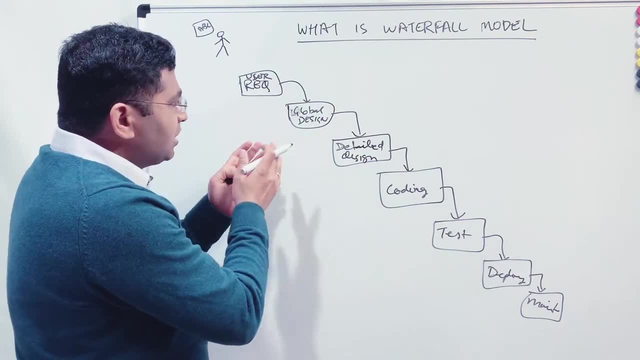 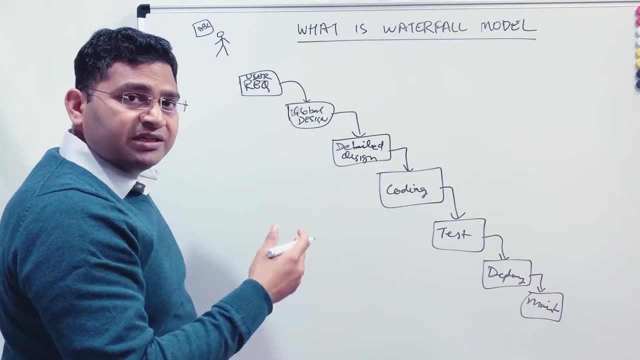 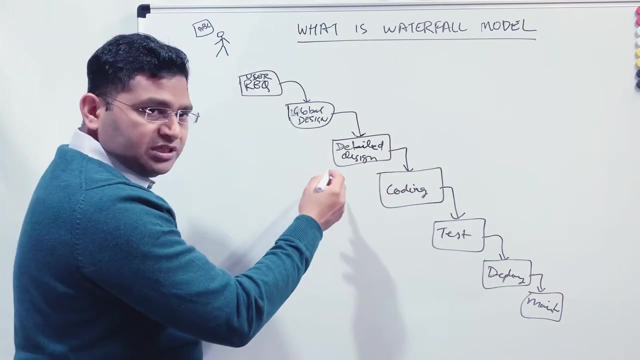 technical architects who will analyze those requirements and they'll develop the or create the global design. Once the global design is being done or completed, only then, detailed design will be starting, or detailed design phase will start. In the detailed design there'll be again detailed. 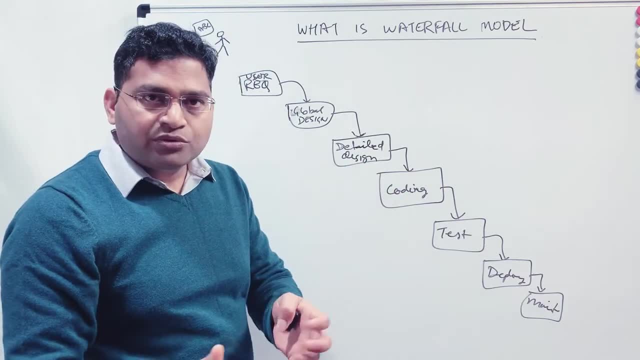 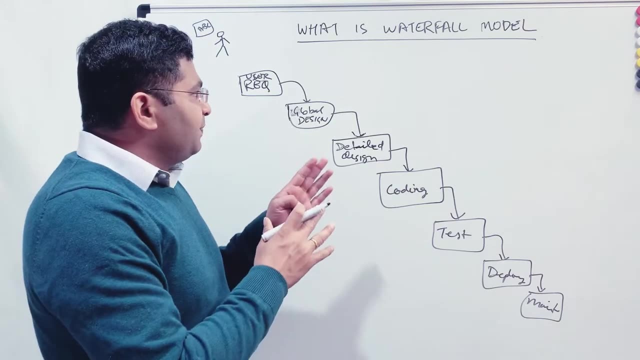 design And, as we see, designing, if you're building a house, you first, you know, gather the requirement how many rooms you want from the customer, right. So if you're an architect, and then where you want the rooms, So 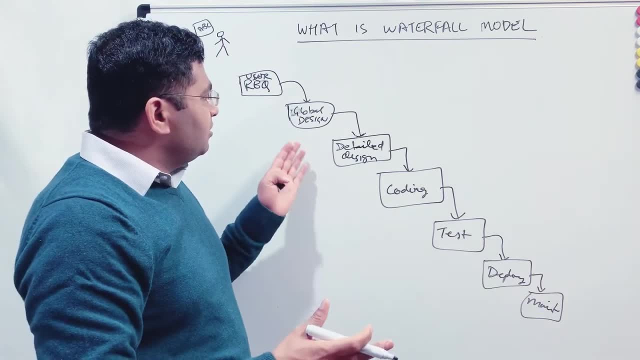 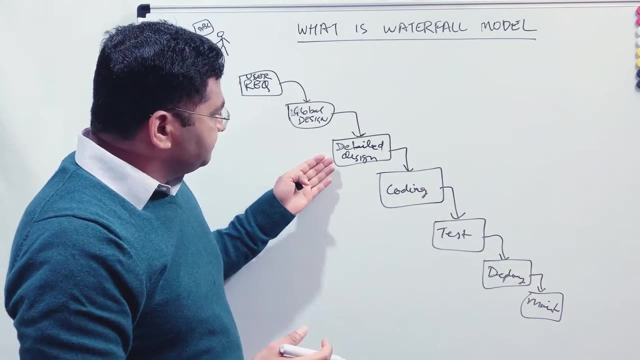 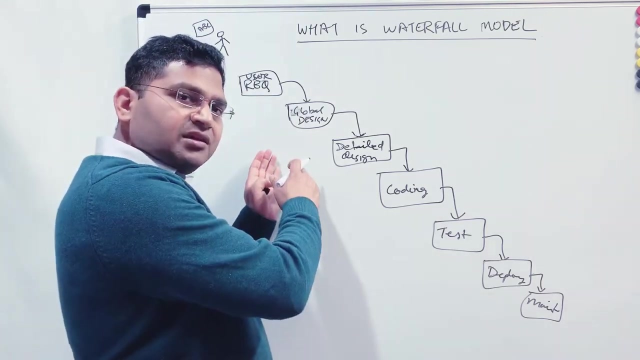 based on that, there is a design being prepared And that design is being shown to the customer that you know. this is what you are looking for, right? So detailed design is being prepared. These are three rooms. there are two bathrooms, you know, kitchen, etc. Similar is the case in the 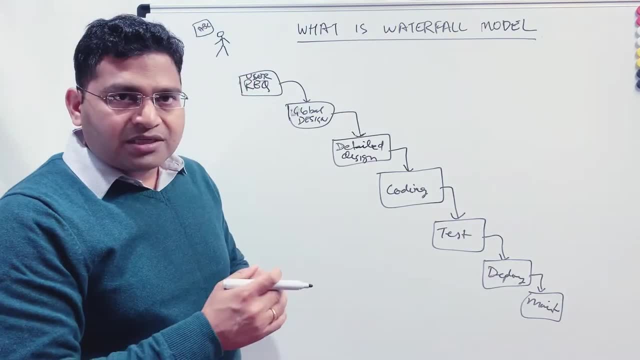 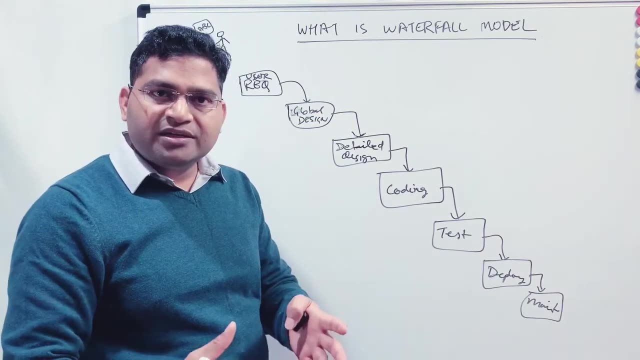 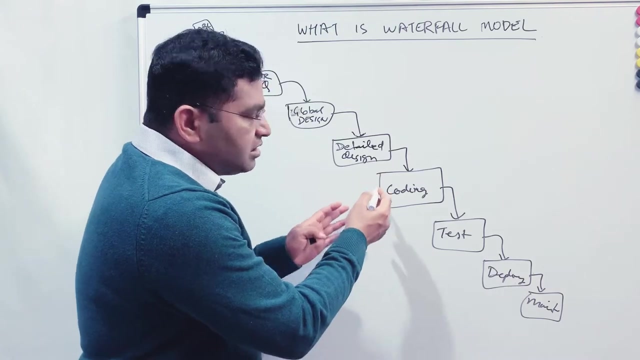 software. Now, once the design, detailed design- is complete, then the team actually starts coding. okay, Similar to house. once the design is ready, you start building the house. you're putting brick and mortar and building the walls right. So similarly in software development, you start coding activity. 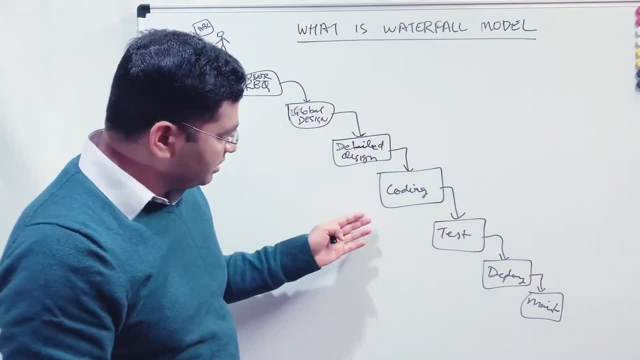 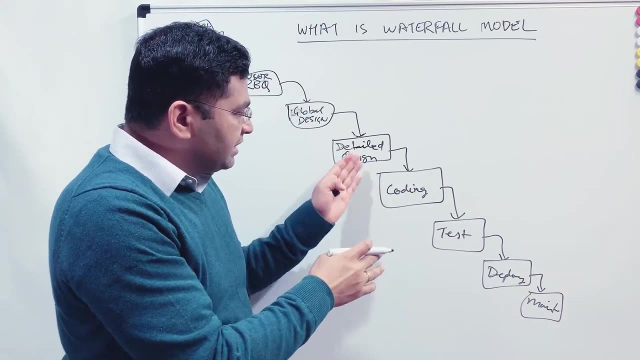 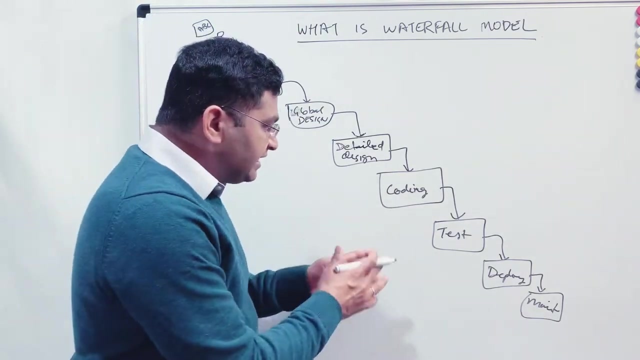 to write the code to build those features. okay, Once the coding is done for all the requirements that have been came from here and designed for that, then the development team moves the software to the test environment, to test team, And then testing starts, testing And 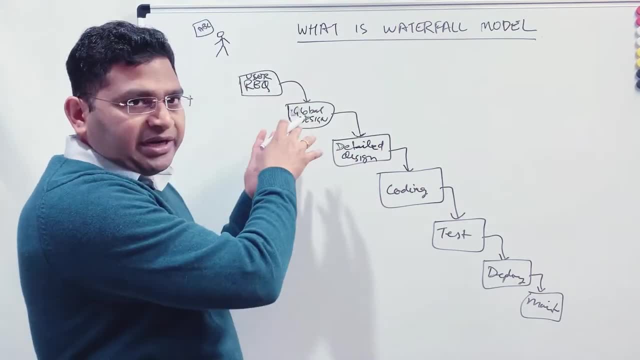 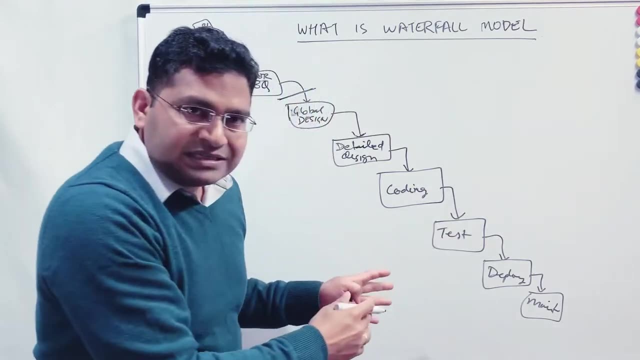 meanwhile they, the testing team, will get their test cases prepared based on the requirements that have been frozen from the requirement phase right. So testing team will start testing, they will execute the test cases and they will raise the effects if the test cases do. 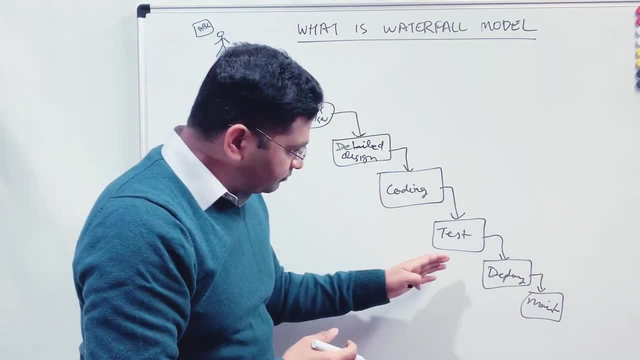 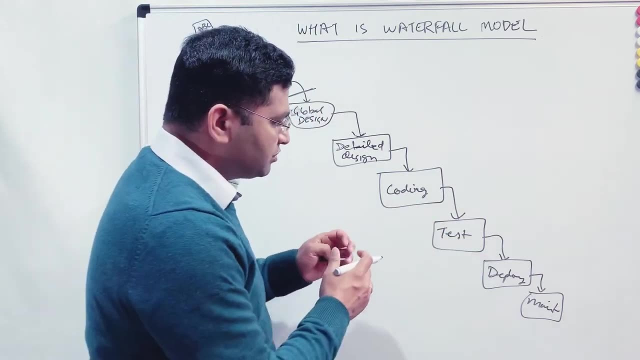 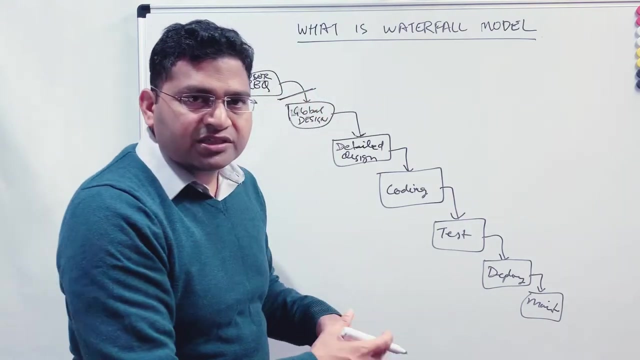 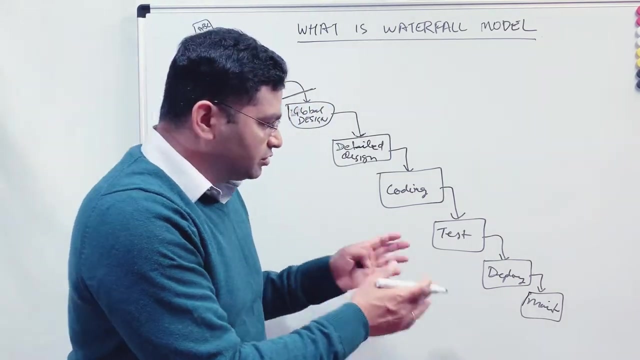 not, you know, fulfill the requirements. After the testing is complete, then the deployment happens of the particular software, so that software is deployed in the production, and after the software is being deployed in production it is available to the customer and then the maintenance team takes over for the maintenance of that particular software. right, 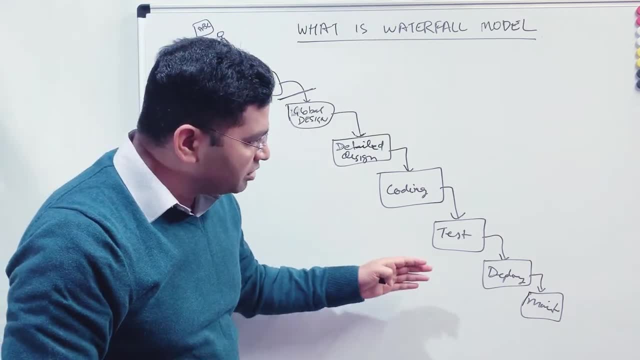 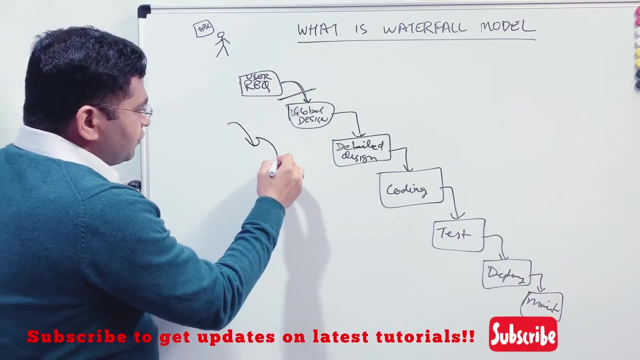 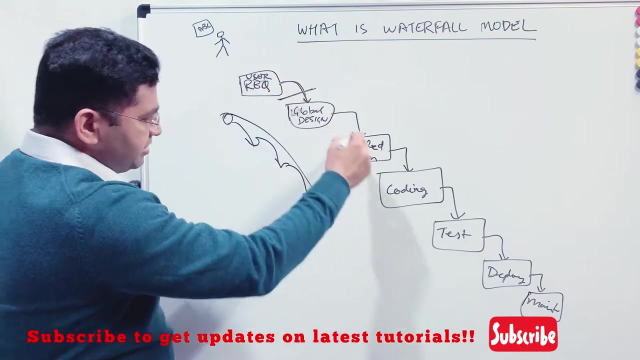 so if you see this particular overall model or process, it follows a waterfall approach. so usually how how water flows, so water flows from top to bottom right. so if, if you drop water from here, it will flow from top to bottom, and similar is the case of the waterfall approach. so there, 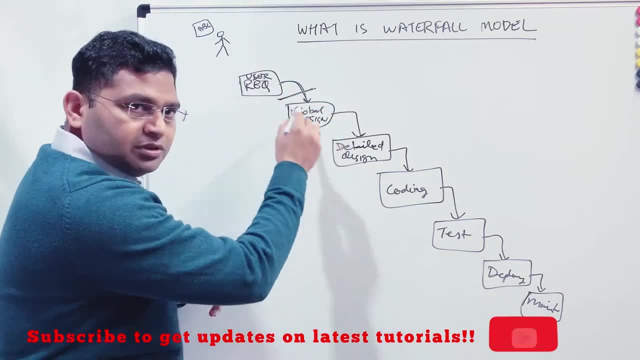 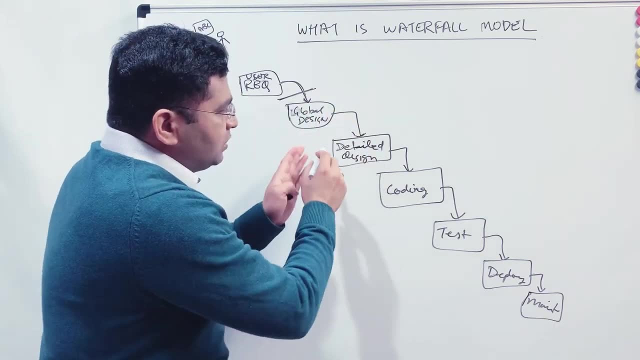 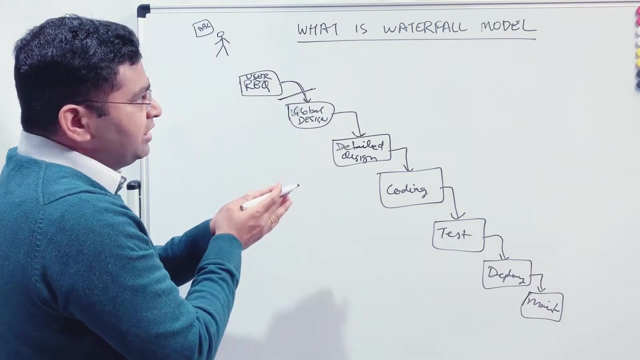 is a user requirement phase. once that is done, then the the work moves to the design phase. once the design is done, then it moves to detail design. once detail design is done, it moves to coding, then testing, then deployment and then maintenance. right, so it is a very, very phased approach and this was the biggest disadvantage of waterfall model. 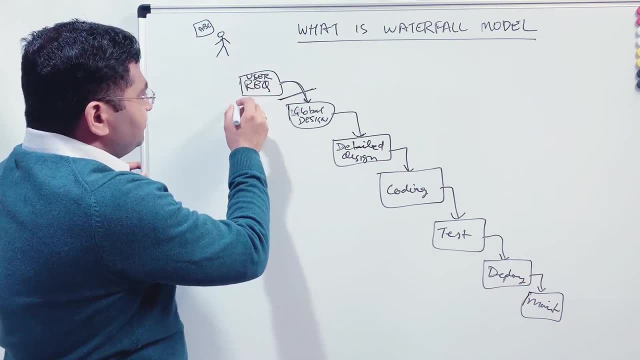 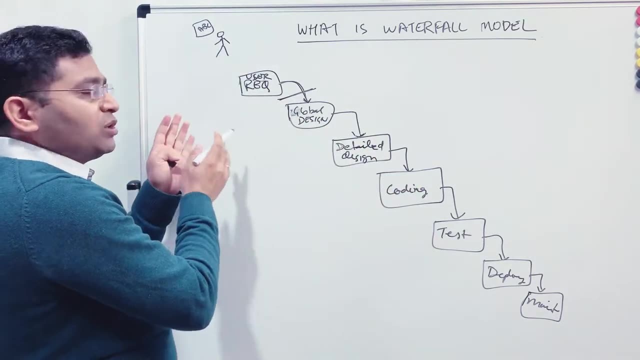 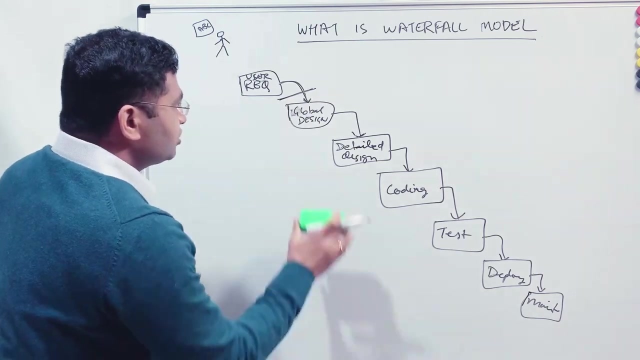 now, if we consider, say, for example, there are issues of gaps in the user requirement which the testing team could have found out if they would have gone through the requirements up front rather than waiting for the requirement until they are frozen right now, because there was a concept of frozen or completing a particular phase before you can move. 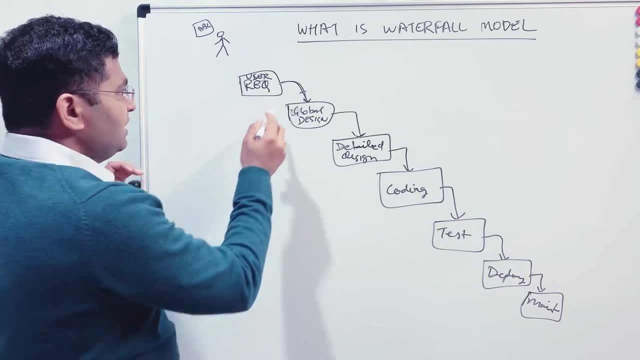 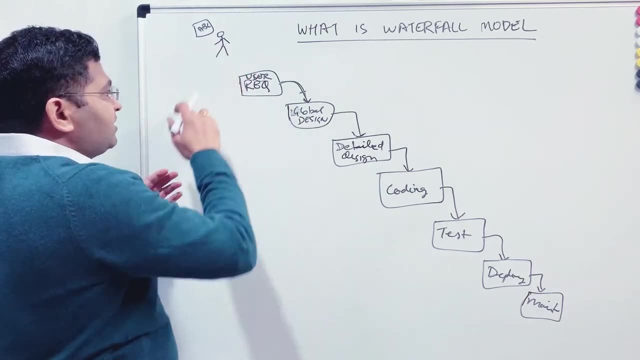 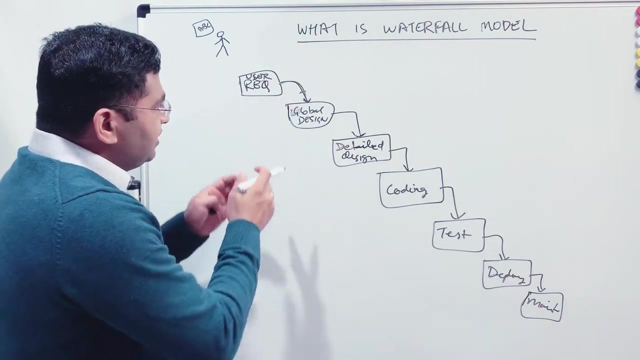 to the next phase. that was another disadvantage in waterfall model. so until the requirements got frozen you cannot start design. and once the requirement got frozen and signed by the customer, that is the source of truth which the whole team or whole process will follow and if, say, for example, there is an issue or gap in the requirement, then design will be. 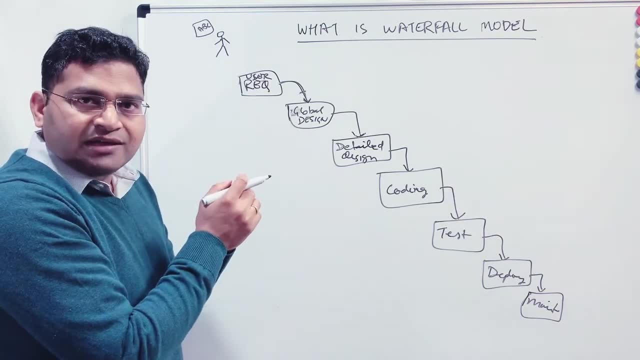 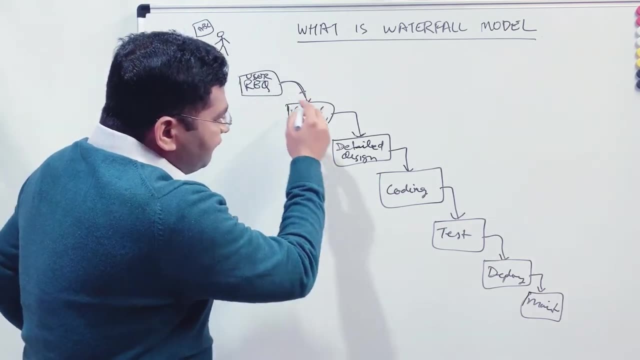 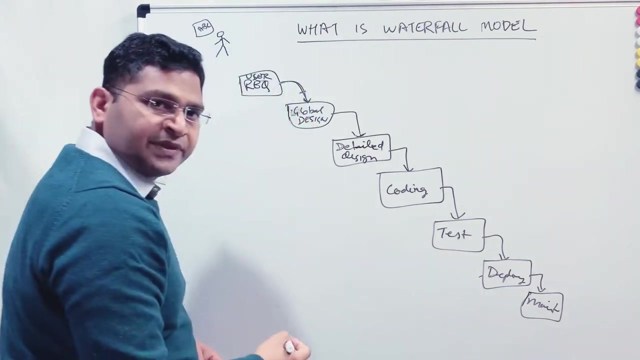 done based on the requirement, whatever requirement is there, and the design will be correct as per the requirement. but the issue is within the requirement, right? so those issues then flow back to coding, testing, deployment and they go undetected until deploy and when you deploy the code, that's. 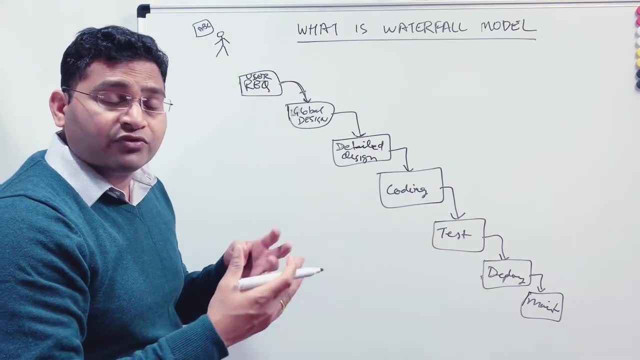 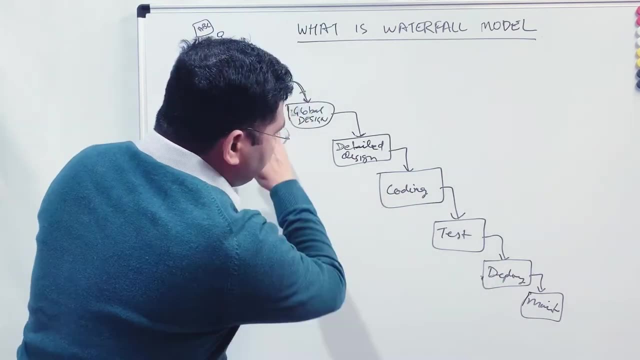 when the customer used to see the working code or working software for the first time, and by the time when he saw the code or the working software it's sort of very late in the life cycle because waterfall approach usually run. we ran from, you know, like waterfall model to rebuilding model. 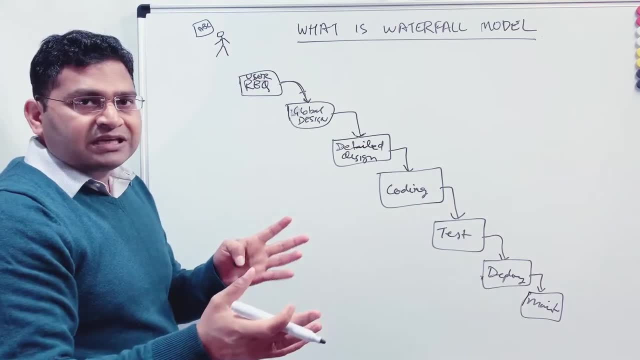 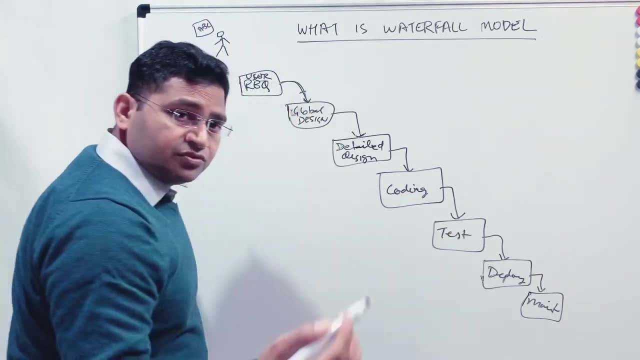 like six months to two years and the releases happen. like eight months or a year after a year the releases happen. so you can imagine like the first deployment or first version that the customer will look like, look or have a look is like eight months down the line or 10 months down the line. 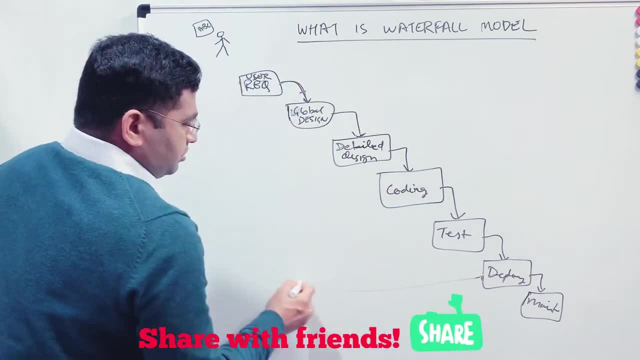 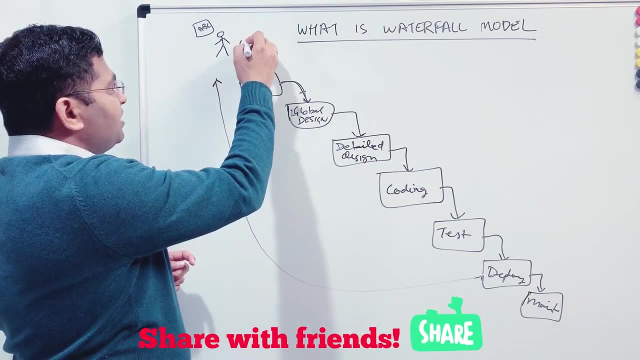 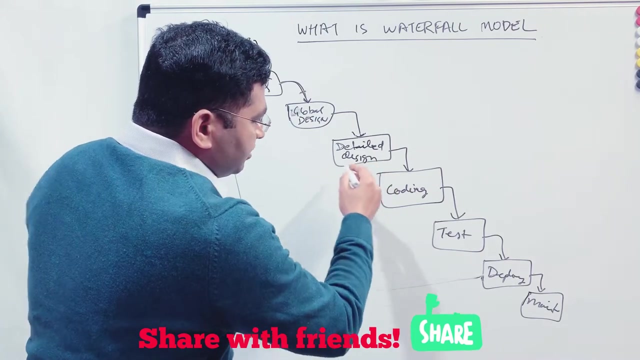 and that's when he'll know that, or that's the you know issue and that's because it was the gap in the user requirement, right? so that will again then come as a change request and change request will be again captured as a requirement and then again it will flow back the coding testing cycle. 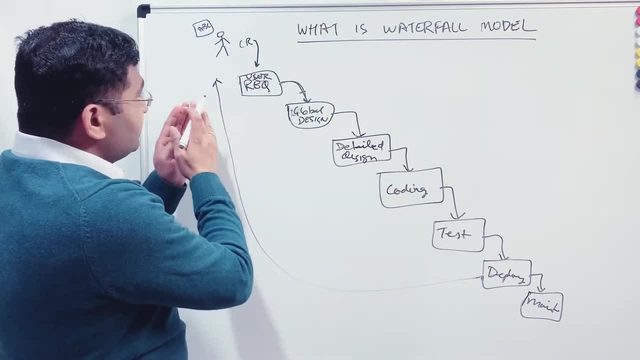 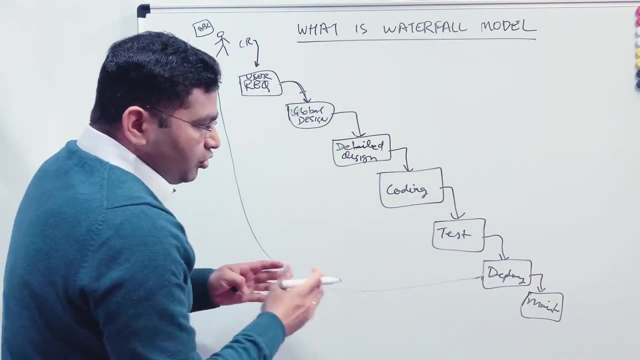 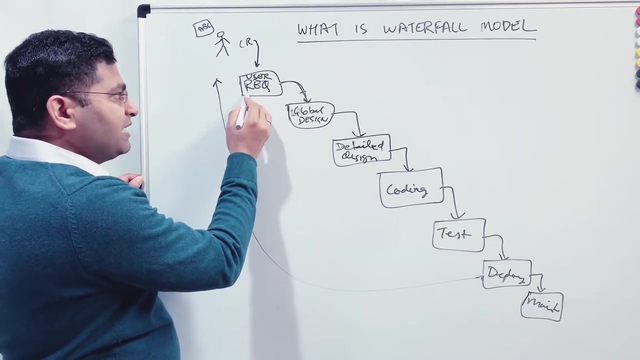 and then it will be fixed and deployed. so this is the biggest disadvantage of the waterfall model, of waterfall software development life cycle. the second thing is basically cost of defect was very high. so now say, for example, there there was a requirement issue which could have been identified here itself if testing team was involved here itself, right? so in this particular 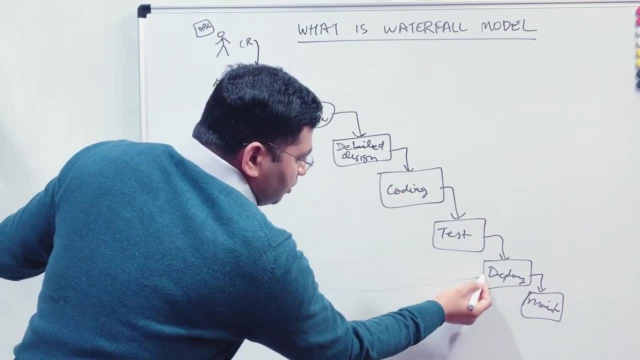 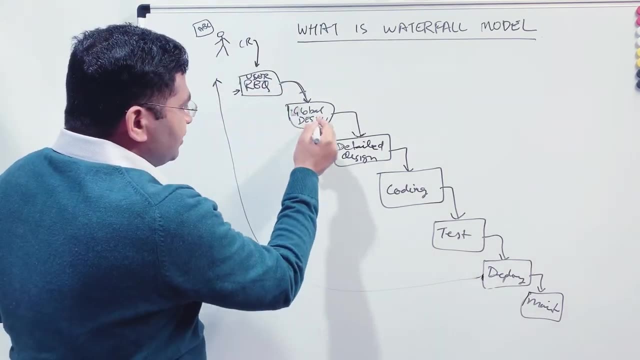 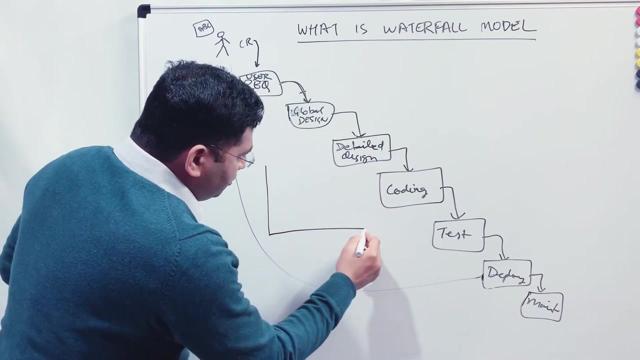 case the issue got found here after the deployment because the issue was with the requirement right. and similarly, if the issue is within the design, then still you know it will be found in the test phase. so all the issues that are found later in the cycle say, for example, this is the 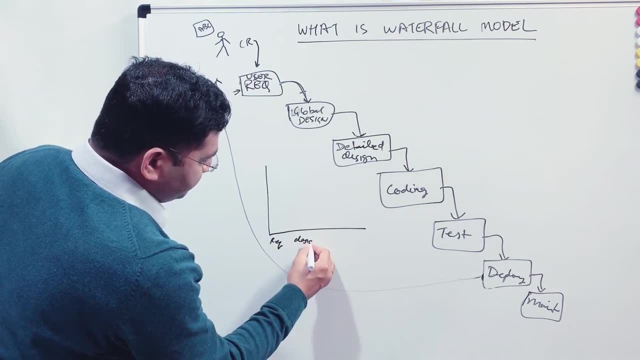 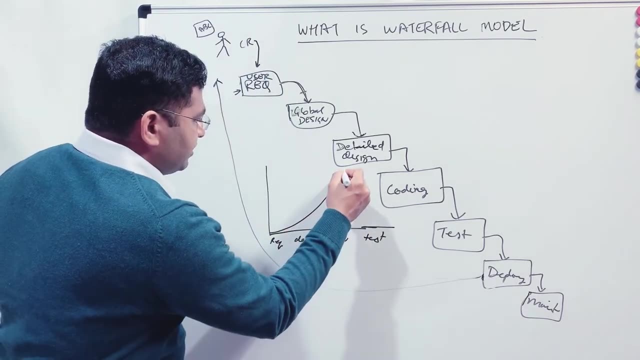 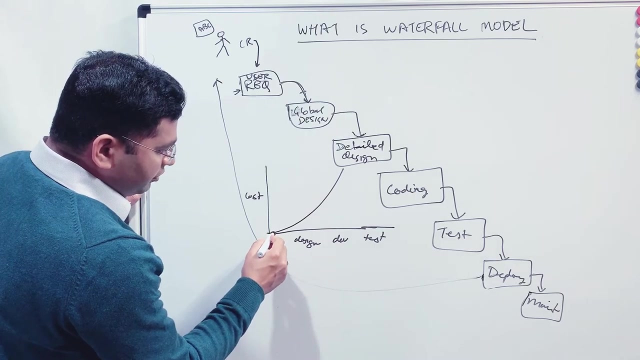 requirement phase. this is design and then develop and then test, right, so you should need to find out, presumaby, the costs of defects. so if there is again, if you see, cost of defect, it is like this. so this is the cost. so if you found a defect in the requirement phase itself, 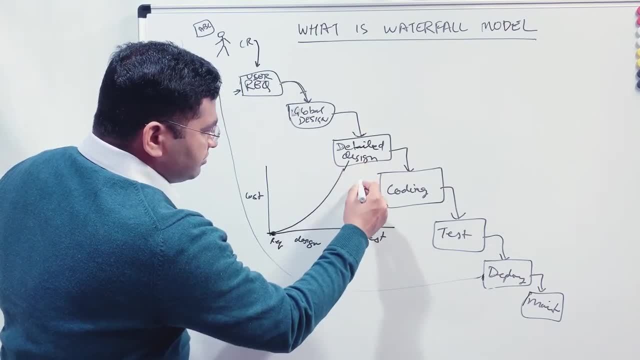 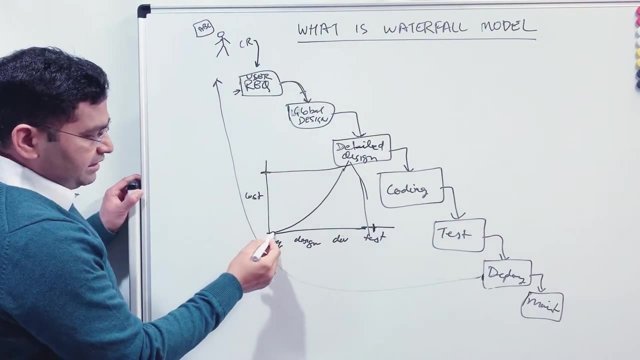 the cost is really low. but if you found it in, you know, like any later phases- say for example test- so the cost is really high. if you see here it will be like this, right, so it's the cost will be here somewhere. and if you found it in the requirement the cost will be really low. so this is why the waterfall approach or the waterfall model was not high enough to face like outside of it and cannot be realised in developing the project within a fixed normal Nebraska. 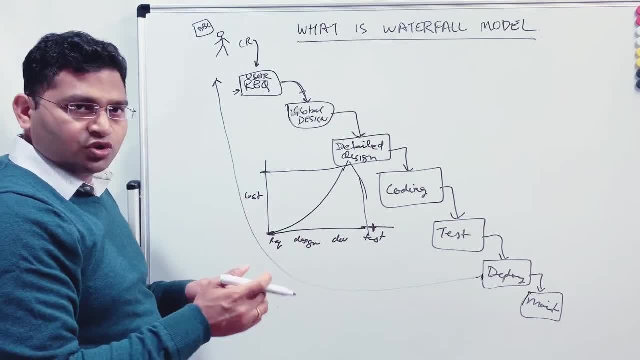 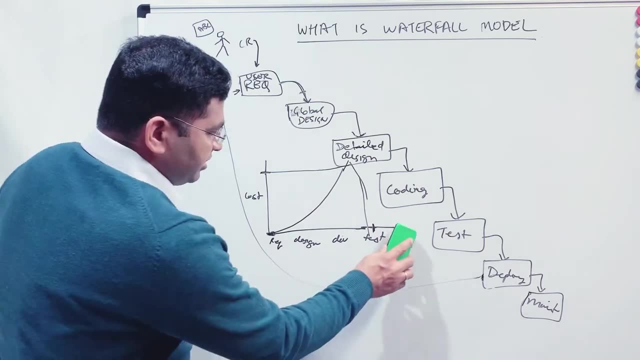 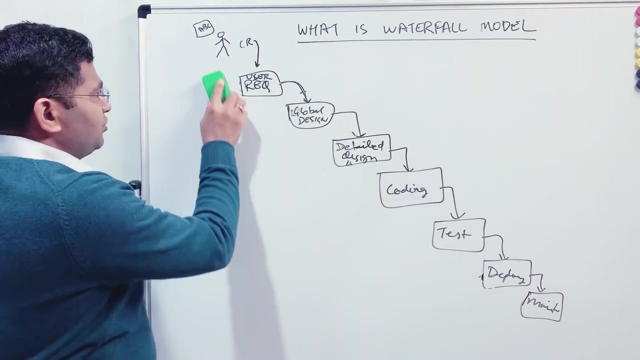 very helpful and that is why the need of change was there, and because of that, there were new development approach that came through, for example, V and agile, which I'll cover in the later tutorials. right, so this is another you know disadvantage of the waterfall approach. now let's understand, you know, say, say.